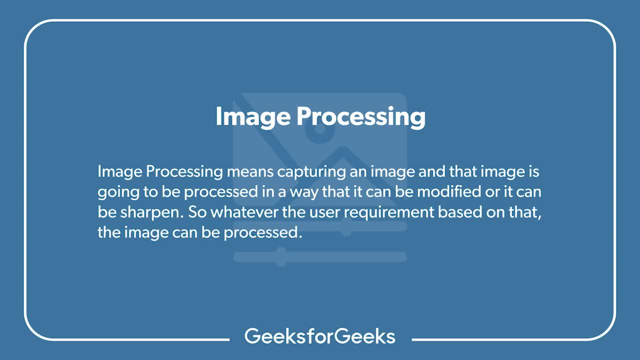 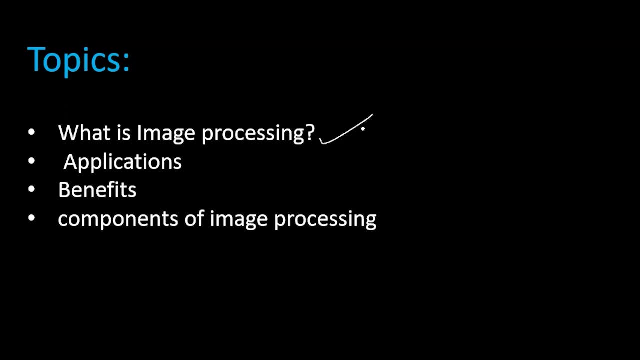 or it can be sharpened. So, whatever the user requirement based on that, the image can be processed. In this video, I'm going to explain about what is the image processing. that is, a definition of image, the different applications of image processing, benefits of using the image. 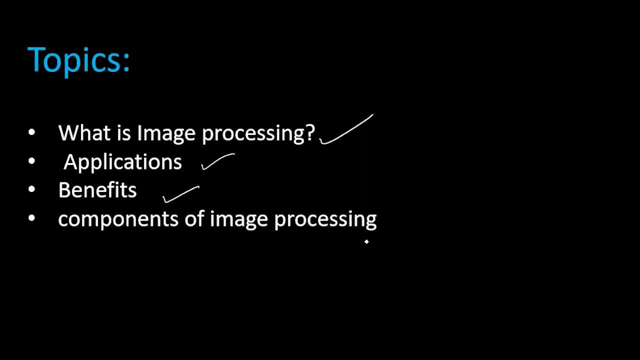 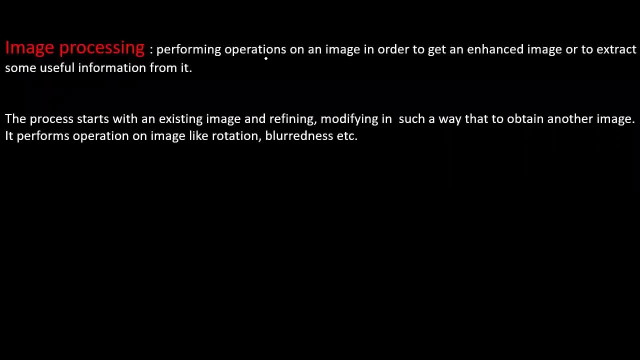 processing and the different components of image processing. Now let's start with image processing definition. Image processing means performing operation on an image in order to get enhanced image. Whatever the image you have taken, that has to be processed and you'll get an enhanced image, or to extract some useful information from it, that you call it. 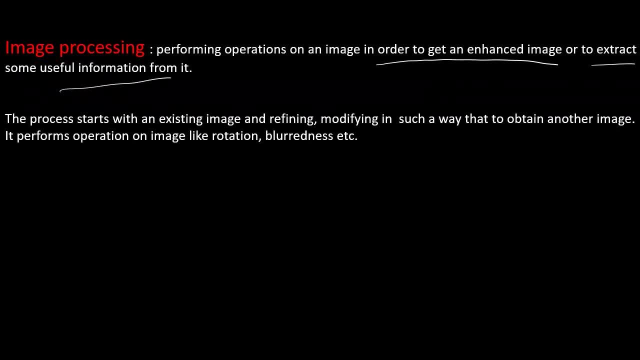 as an image processing. Okay, let me give a clarity by taking a live example. Suppose, if you see the flex board, what you'll do your first. your eyes will first capture the board- the flex board- and your brain will process it and it is decide whether this is an exact shop that you're. 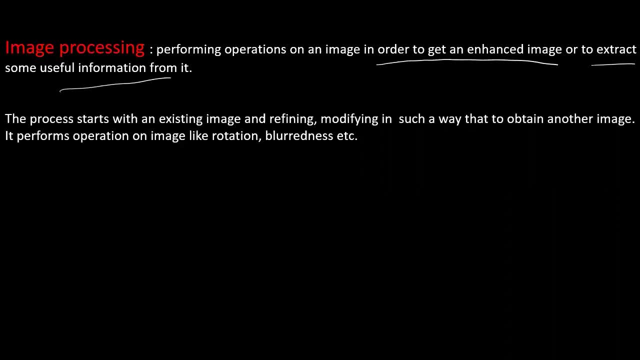 searching or not. Right Means here what happening. image is a flex board and your eyes are capturing that image and your brain is processing it and it is giving a conclusion whether this is exact shop or not. So it is a human If you consider the image processing in the human. in the same way, suppose if you take the 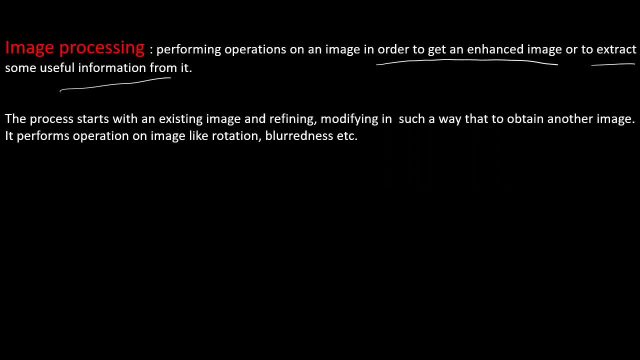 traffic signals. whenever your eyes is going to capture the green light So, and your brain is processed it, then we will start moving whenever the green light is appeared. So that is image processing. while we are talking about the human being, human being processing, capturing, is through. 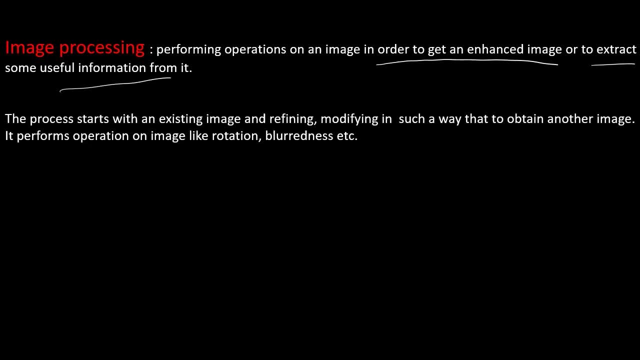 eyes And processing through brain. in the same way, The image is captured. If you talk about in the techno, technical terms, the image is captured through camera. Okay, with the help of, suppose, the camera is there. So, with the help of the camera, images capture and inside the system, with the help 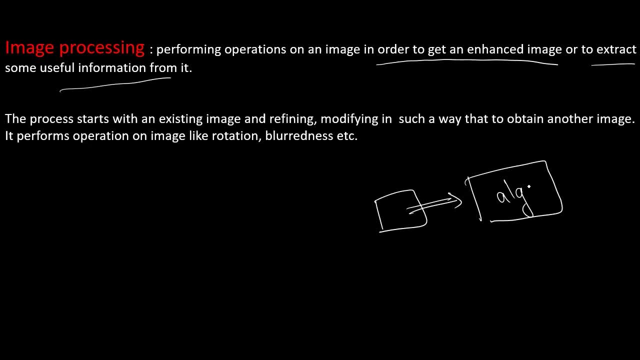 of some algorithms. we are modifying that, refining that and whatever the image that you want- enhanced image or extract. If you want extract Some useful information on that picture- that, whatever the user requirement, the output will be appeared. Okay, so what this image processing will be doing? the process starts with existing image. It just take an existing. 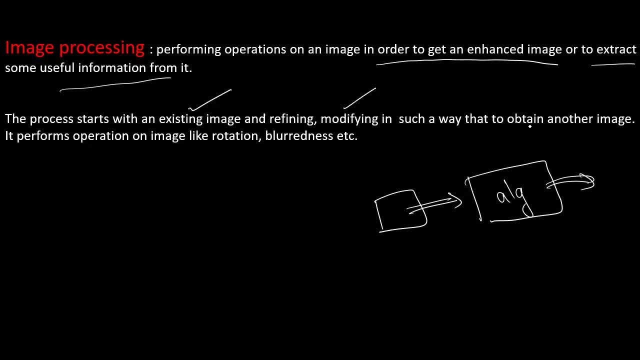 image and refining, modifying in a such a way that to obtain another image. It performs operations on images like it will do rotation. It can make it as a blurriness, It can create a sharpness Images, so different operations It can be performed. 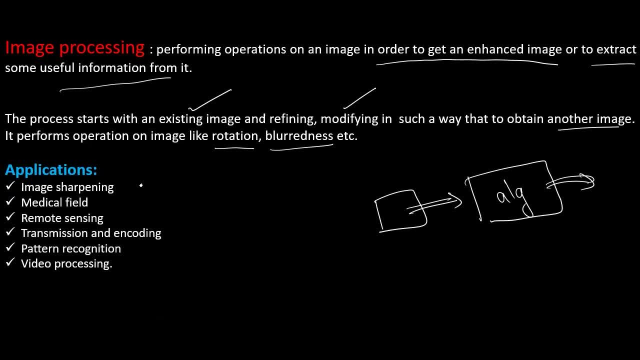 Now let's have a look on the applications of image processing. image sharpening We are going to use in the medical field. Image processing is used in the medical field: remote sensing transmission and encoding pattern recognition video processing. So these are all the different areas where the image processing is used. 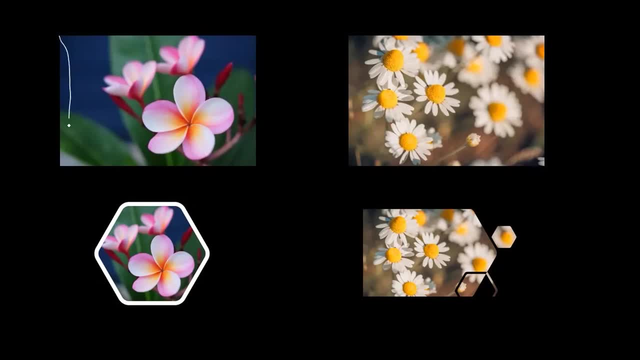 So here, if you see this picture, let's capture an image. So this is a Complete image that we captured. If you want a detailed study about a small flower, you just capture only that picture and you can refine it and you can create a. 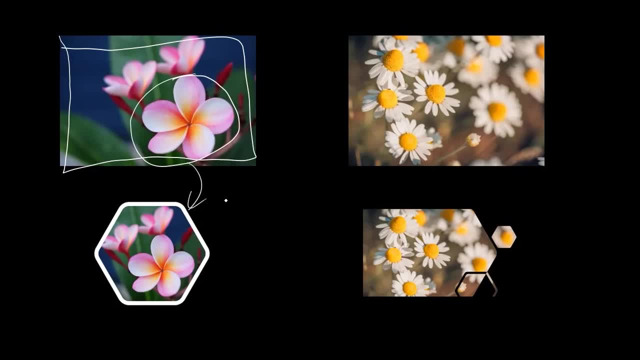 modifications on that. Okay, so this is a way of image processing: Capturing the image and processing whatever you want. you can make the complete background as a blurred and you can take whatever the information that you want. You can extract the information, what you, whatever you want, with the help of this image processing. 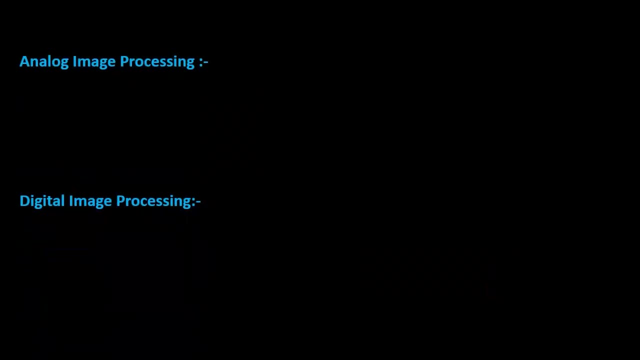 Now coming to the next concept, the analog image processing and digital image processing. Actually, there are two types of image processing. Either you can perform in analog mode or in it in a digital mode. So what is this analog and what is a digital? 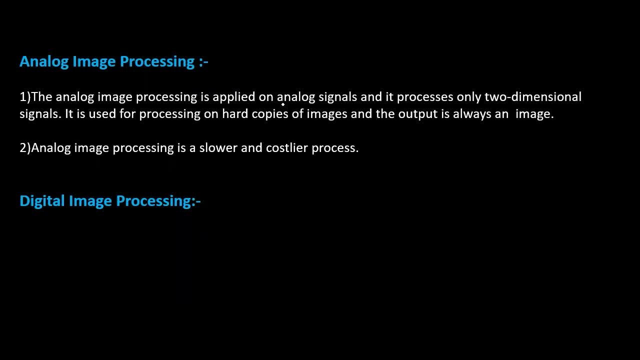 Let's have a look. The analog image processing is applied on analog signals And it process only two-dimensional signals. and the main use of this analog image processing is on hard copy of images. means you just take a hard copies, like x-rays, and you can take the print out. 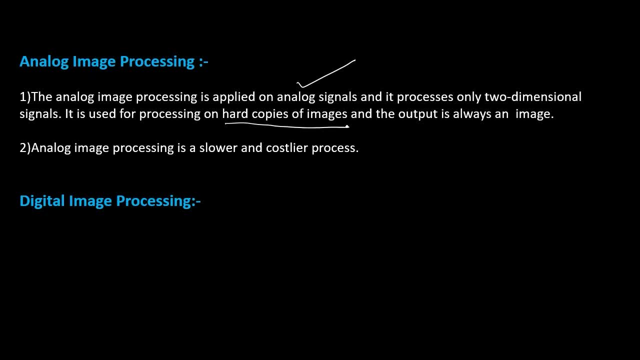 So on that only the analog image processing can be applied and the output is always an image. Whatever the image you are captured, the output will be that image only. analog image processing is slower and costlier processor, So that's why mostly we go waiting. 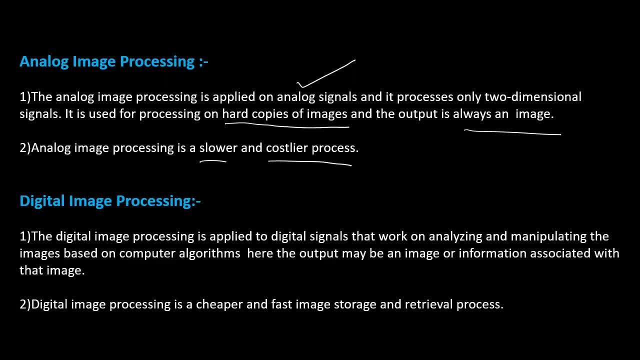 We are not preferring To use analog image processing. We always look about the digital image processing. Nowadays, the complete world is concentrating on and using the digital environment only. So what is this digital image processing? The digital image processing is applied to digital signals that work on analyzing 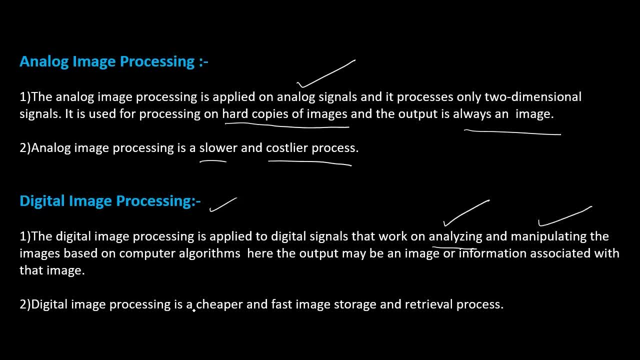 What is it doing? It analyzing, manipulating the image based on computer algorithms. with the help of the computer algorithms, Only the image, digital image- is captured Through cameras, Okay, and it is analyzing and manipulating and the output may be an image or it can give some useful information associated. 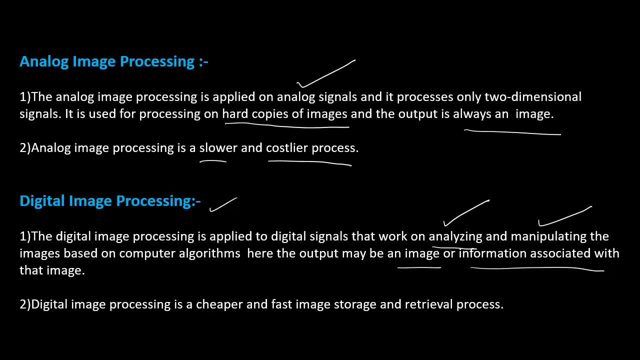 with that image. It is not compulsory. Every time it will give only the output as an image. but in an analog image processing the output is always image. but in digital image processing it is not only the image but it can give the useful information regarding that image also. 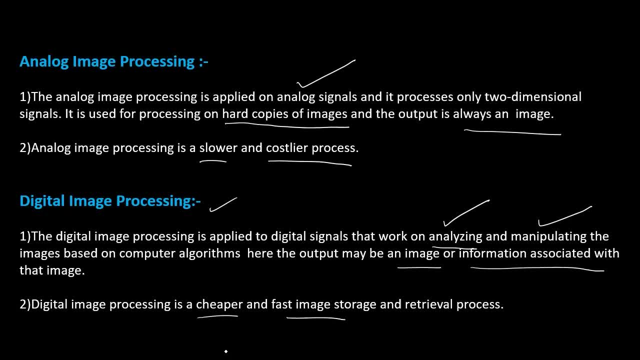 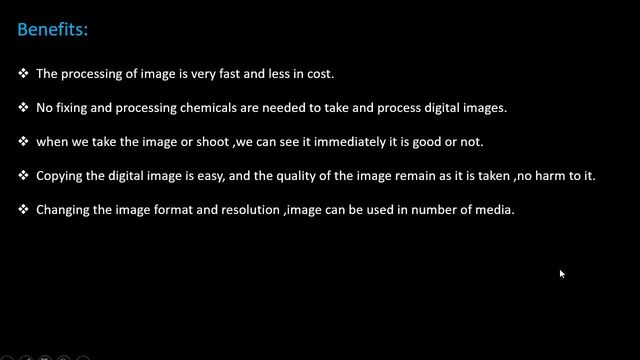 digital image processing is cheaper and faster image storage And retrieval process. So that's why we are using digital image processing nowadays, Now coming to different benefits of using the image processing. the processing of image is very fast and is in less cost, Obviously so because of that, only nowadays everyone is focusing and using this digital image processing. because the processing of 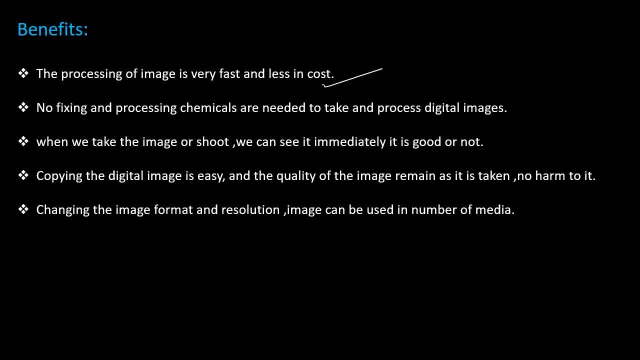 image is very fast when compared to the analog also, and it is less in cost. Also, There is no Fixing and processing chemicals are needed to take and process digital image Simply. you can capture the image. how many images that you want you can capture. 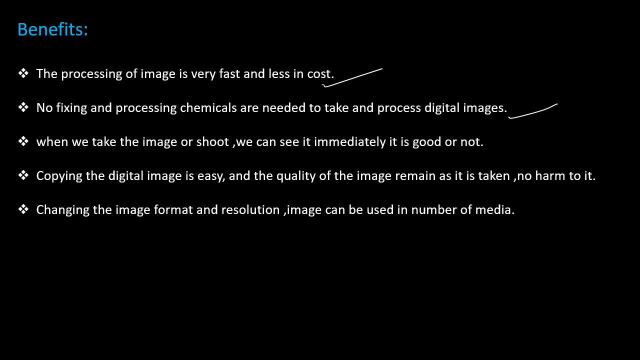 There is no need of fixing anything and that you don't require any chemicals to process them to capture the image. When we take the image or a shoot, we can see it immediately. It is good or not, and seeing the camera you are just finding and you are just looking that, whether the you got the picture, clarity or not, everything. 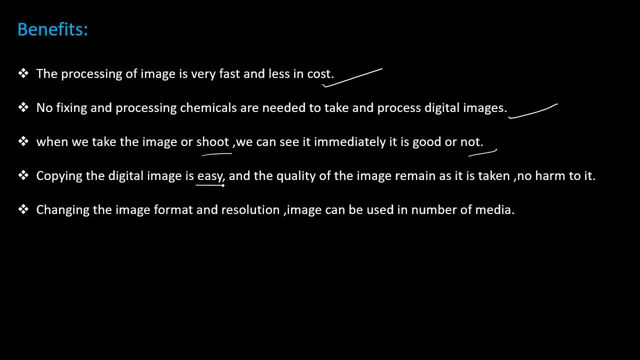 So it is very easy. Copying the digital image is easy and the quality of the image remains as it is taken. no harm to eat, So the quality is also superb and, at the same time, if you want to copy the digital image, it is very easy. 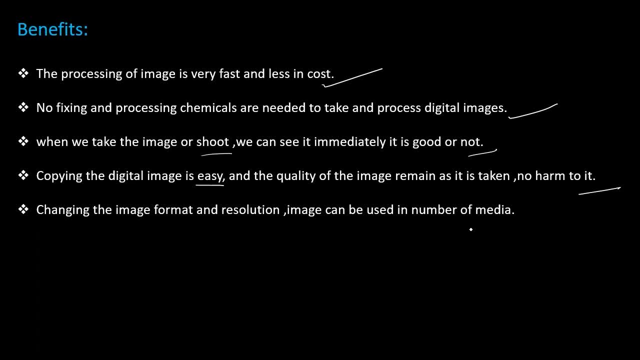 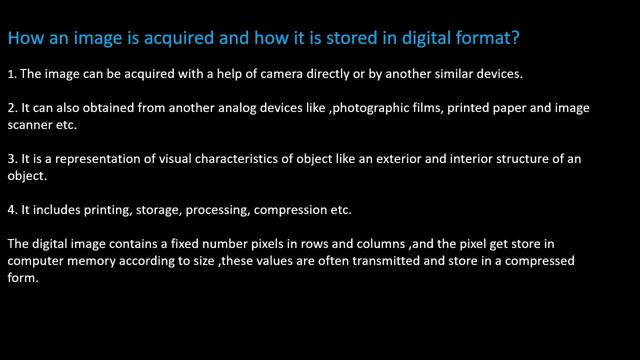 Changing the image format and resolution. image can be used in number of medias. Now There is a doubt how an image is acquired and how it is stored in digital format. So everyone is getting a doubt How these images are acquiring and how we are going to store in the digital format. 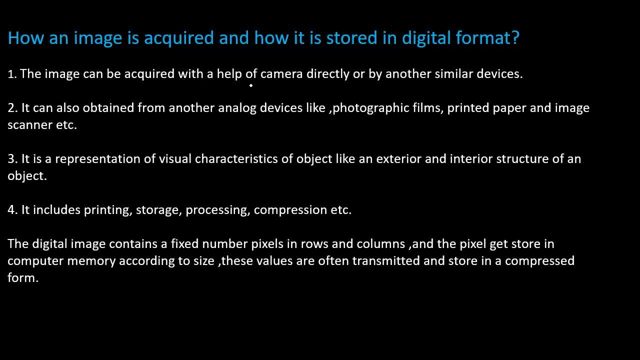 Let's have a look here. The image can be acquired with the help of a camera, directly or by another similar devices, Not only camera. You can take your mobile phones, You can take any shooting devices, anything, so you can capture that image with the help of that devices. 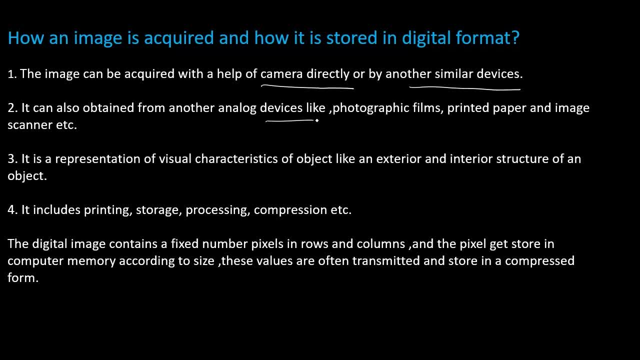 First thing. next, it can also obtain from another analog devices like photographic films, printed papers, image scanners. So not only in digitally, you can also captured by analog. It is representation of visual characteristics of objects, like an exterior and interior structure of an object, And it also includes the printing, storage, processing, compression, Etc. 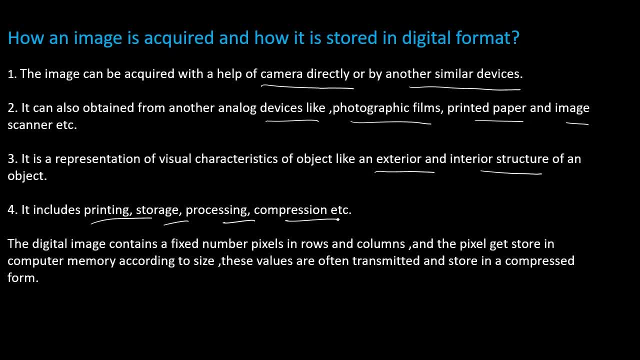 So, if you talk about the digital format storage, the digital image contains a fixed number of pixels in rows and columns. This is already I discussed whenever I talked about the pixels. The digital image contains a fixed number of pixels that is arranged in rows and columns and the pixel gets stored in computer memory according to the size. 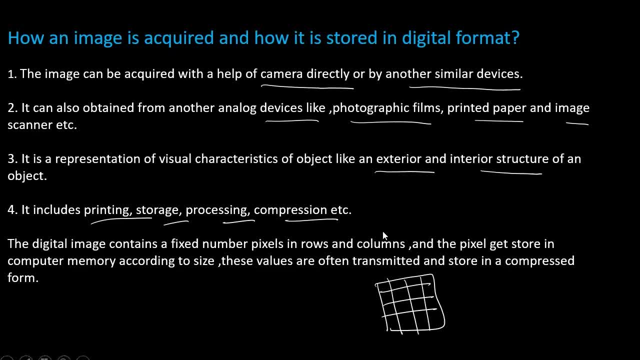 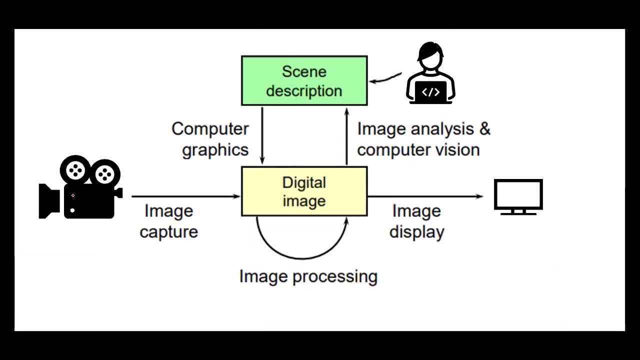 These values are often transmitted and stored in compressed form. So see here This is a capture, digital image, image capturing, Okay, and here image display. that is the output screen. So whenever the image is captured, that Sent into the computer or any electronic gadget for processing that image. 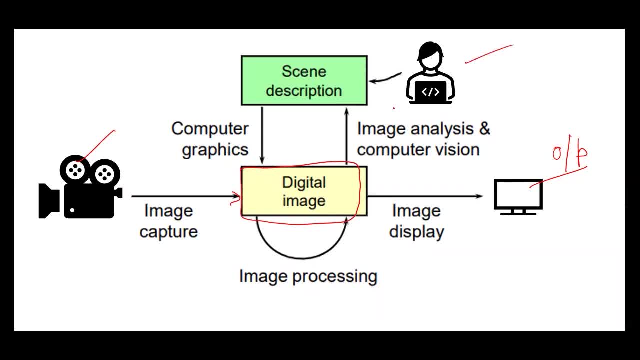 This is the digital image. So here the user, the person who is going to modify that image and his image analysis and computer vision. with the help of a computer graphics, It sends the data here and there is image processing. The final output is going to be displayed on image display. 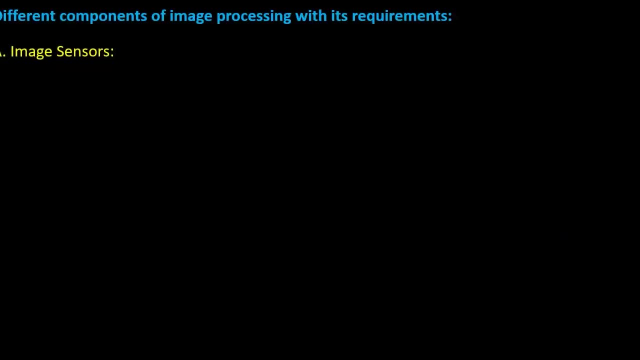 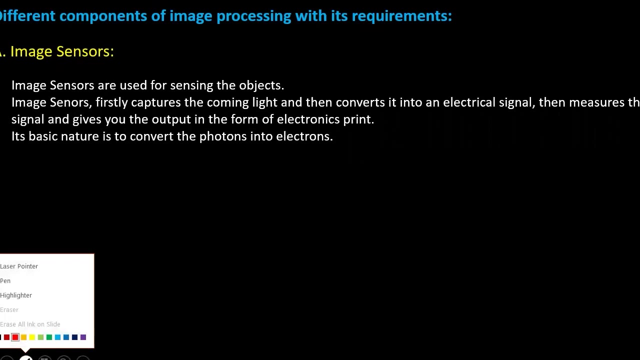 So now, coming to different components of Image processing, with its requirement, The first component here I'm talking about is image sensor. So what is this image sensor? image sensors are used for sensing the objects. The first, first component in image processing is first: 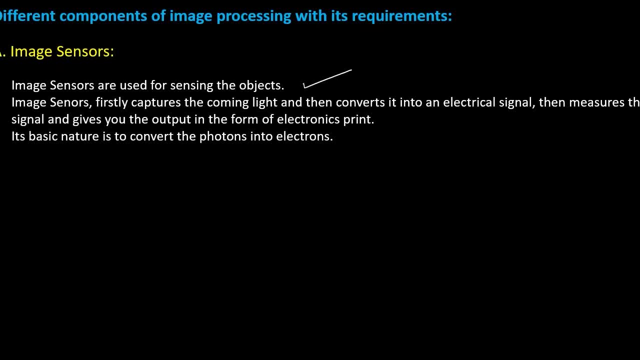 You need to sensor the object. If you want to capture the object first, you need to sense it right. So image sensor used for sensing the object. image sensors firstly capture the coming light And then converts it into an electrical signals, Then measures the signals and give you the output in the form of electronic print. 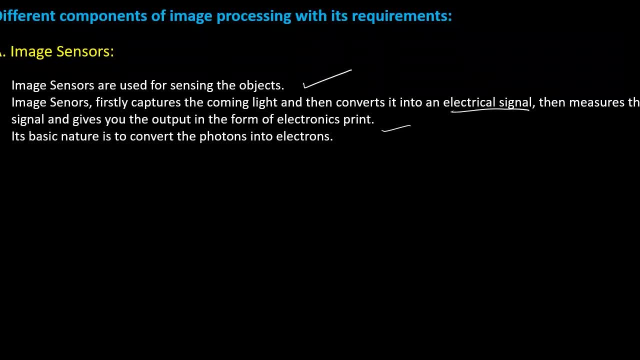 So it's basic nature is to convert the photons into electrons. That is image sensor. And coming to the next component, that is the hardware of image processing. Okay, what type of hardware you required for image processing? It is a hardware that performs the arithmetic logic unit, which is used to perform some 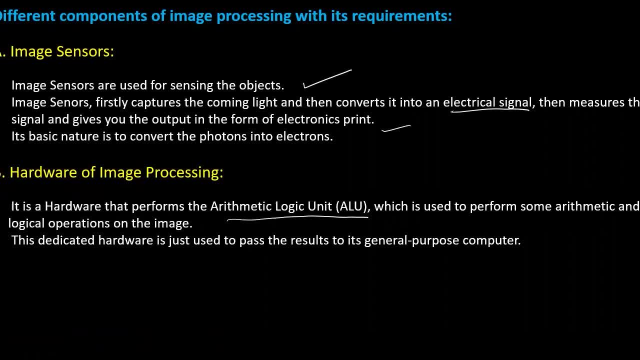 Arithmetic and logical operations on image. So if you take the image, it has to perform some arithmetic and logical calculations: means the pixel should be added, The pixel should be removed and how much quantity you need to be added so that the sharpness will be appeared. 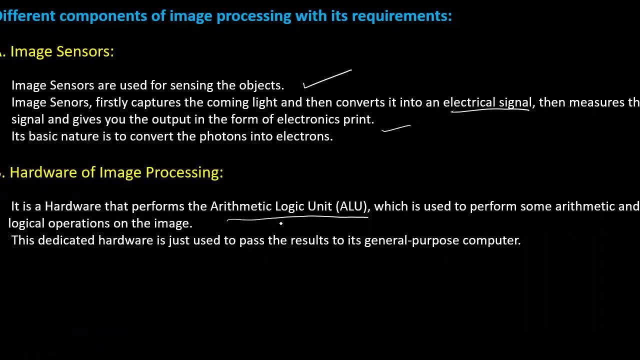 So like that. so it has to be performed on arithmetic logic unit. This dedicates hardware is just used to pass the result to its general-purpose computer. and the third component of image processing and its Requirement is computer or a PC. You required it to perform an operation. 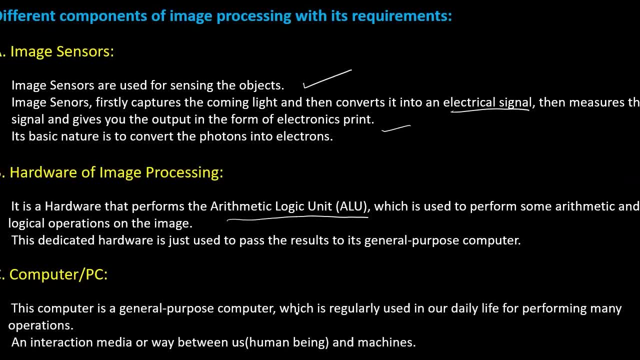 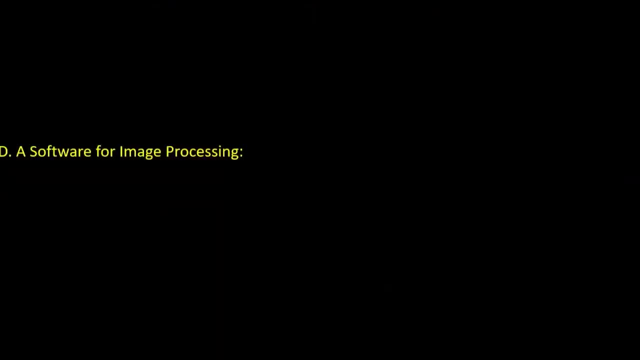 You required something right. So this computer is a general-purpose computer which is regularly used on our daily life for performing many operations, Just like your laptops, your tablet, anything, and interaction media or a way between human beings and a machine. The next component is a software for image processing. a software is a machine inner tool. 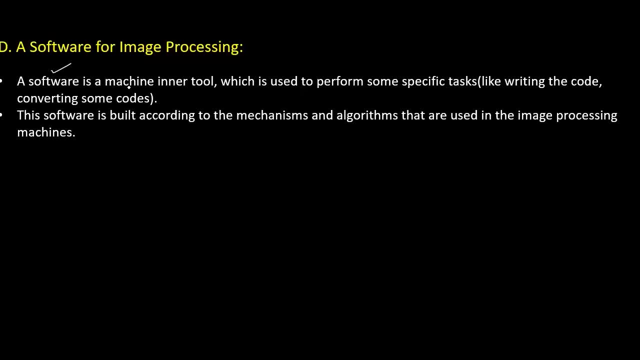 Remember, student, whatever the software we are taking, that software is a machine inner tool Which is used to perform some specific tasks, like writing the code, converting some codes. So this software is built according to the mechanism and algorithm that are used in the image processing machines.